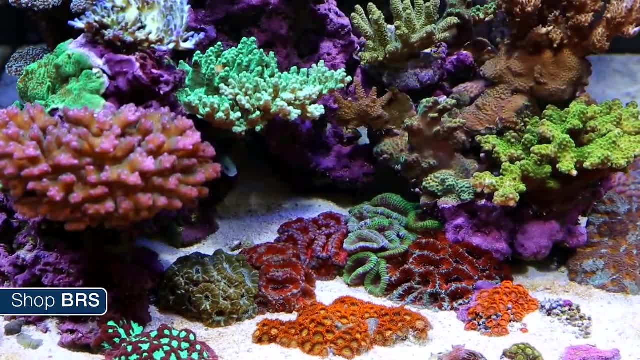 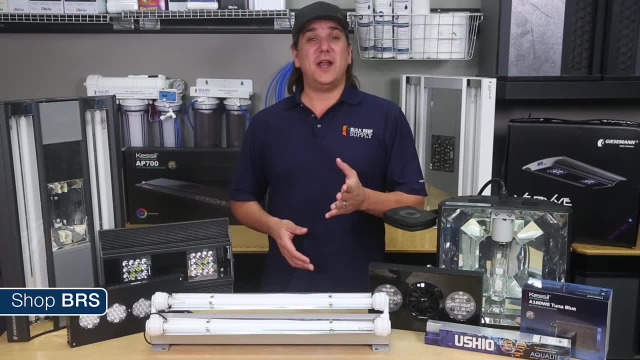 And that's the ability to produce light, Light intensities and wavelengths that promote photosynthesis and, in turn, produce nutrients which feed the coral's metabolic system, health and growth. So if there's only one element, the reefing community needs to evaluate every light source. 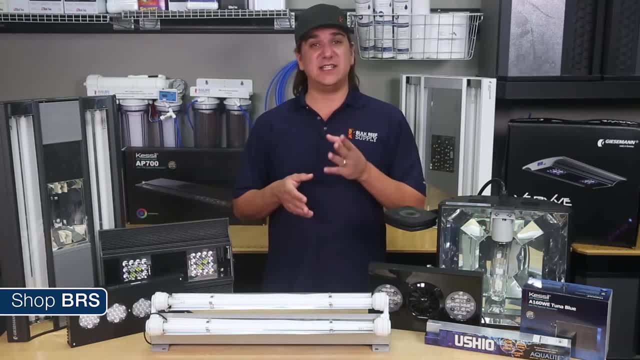 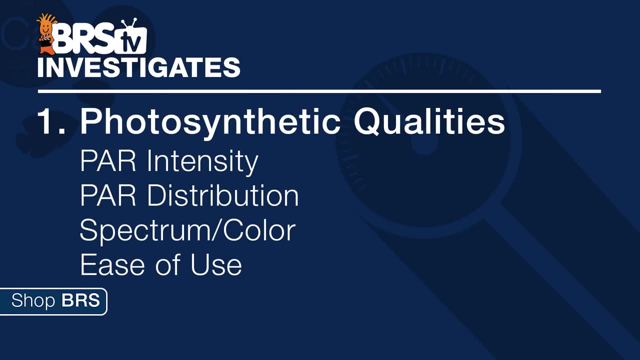 for it's absolutely photosynthetic qualities of that light and I can tell you for sure, while most will work to some degree, they're all very far from the same in terms of four major elements: PAR intensity, PAR distribution or spread of that intensity spectrum. and 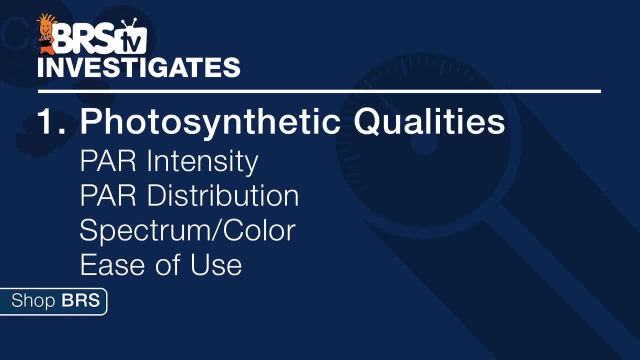 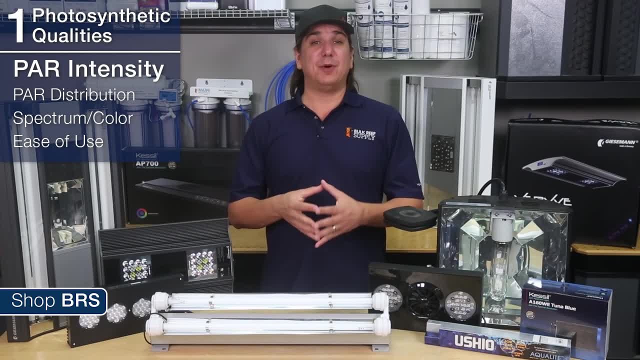 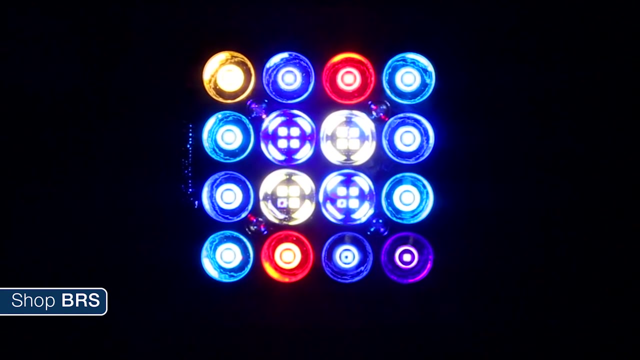 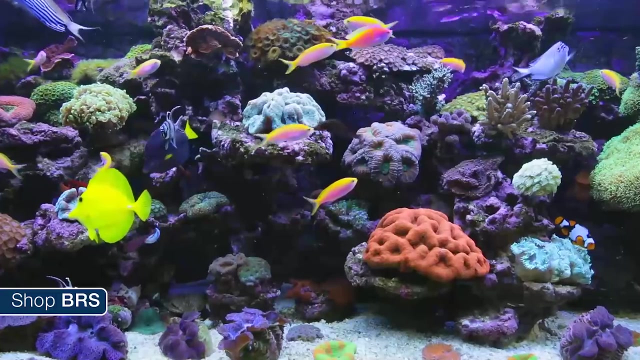 color and how easy it is to use the light source to achieve photosynthesis. Thanks for watching. I hope you enjoyed this video and I'll see you in the next one. Bye, bye, Bye. And now I'm going to finish up this video with this key feature, which I found to be: 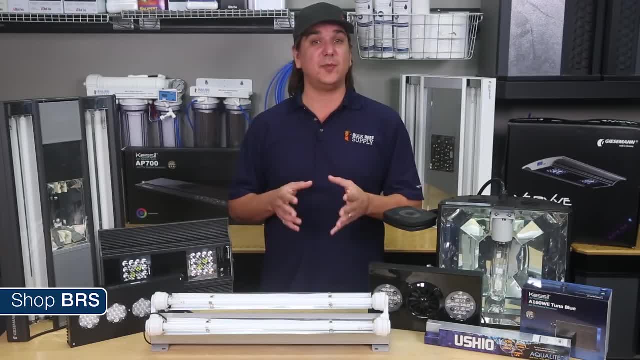 many of the most important elements of this new technology, and yet it's probably one of the few that truly needed it. So manufacturers produced them, and it became one of the most defining characteristics or marketable elements between all the lighting options. And so the PAR wars began, with one manufacturer constantly trying to produce higher PAR numbers. 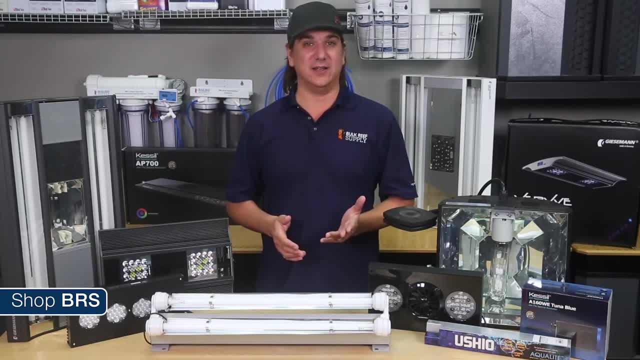 then the next, because that's what the market demanded and wanted to buy. At this point, some of the lights are producing peak PAR numbers close to those found at noon near equatorial shallow reefs. At face value, that might sound good. however, a lot of reefers just end up killing a lot. 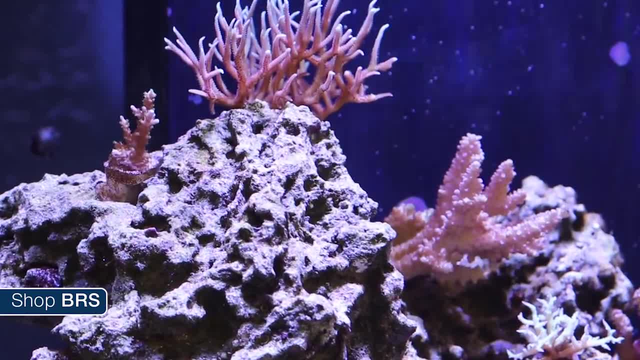 of expensive corals when they try to implement those levels in a reef. Well, I've known a lot of reefers who are excited to try out some of the best lights. implement those levels in a reef tank environment. The presumption that natural reef peak mid-day levels are desirable- your particular corals. 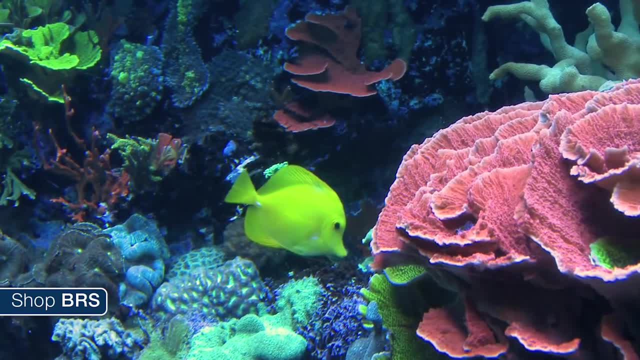 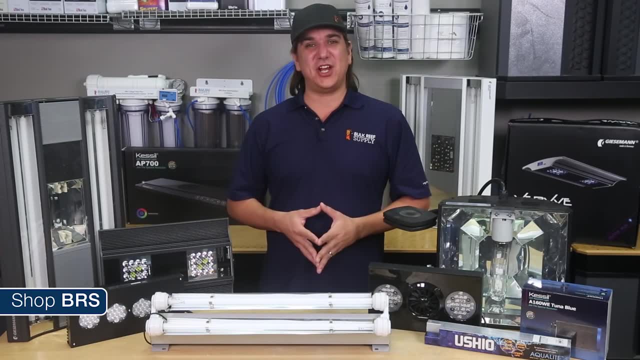 came from an area or depth with those PAR levels and your system has similar flow or other environmental characteristics, is a major stretch. Just to give you an idea why that is almost certainly not the case, I would like to share some info from Dana Riddle's presentation at last year's MACNA. turbocharged photosynthesis. 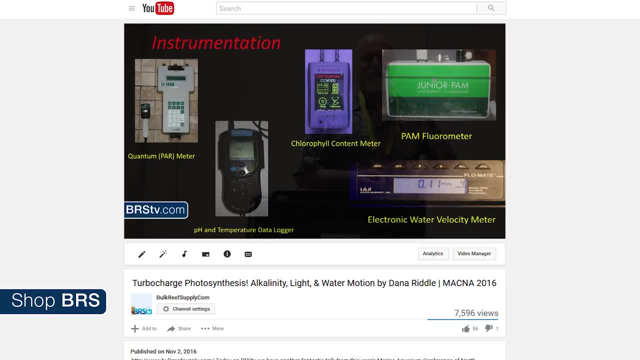 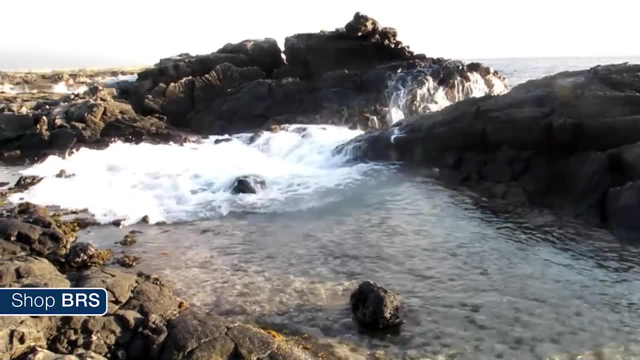 alkalinity, light and water motion. If you haven't watched this, we have the entire presentation on our YouTube channel and it is well worth your time. In this presentation, he measures a tide pool in Hawaii which, during mid-day, approaches a thousand PAR at two inches of depth, which is somewhat similar to some of the LED aquarium. 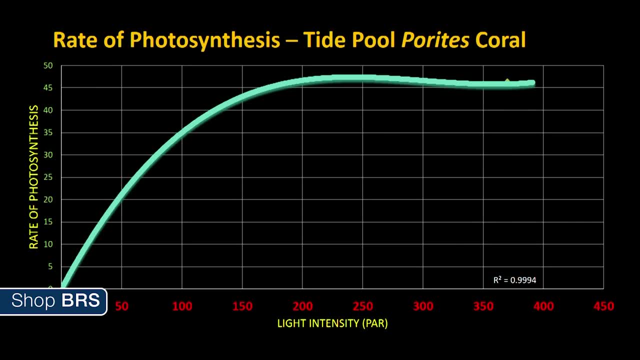 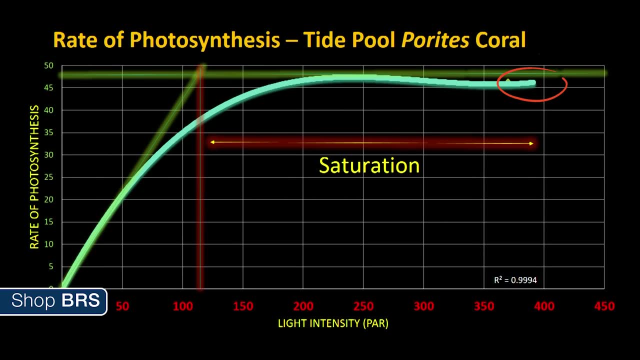 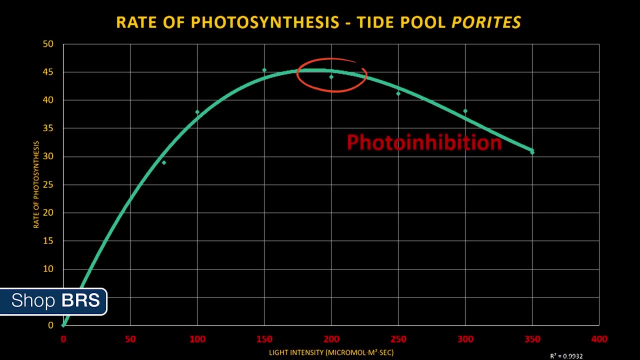 lights output. However, he also measured the rate of photosynthesis of a parites coral living in that pool and found a very limited difference in photosynthesis between 120 and about 400 PAR, and at 250 it seemed to drop off. With another specimen, the photosynthesis starts to slow down rapidly after 200 PAR, so even 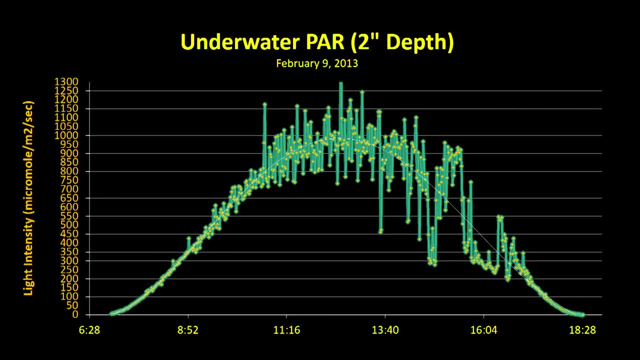 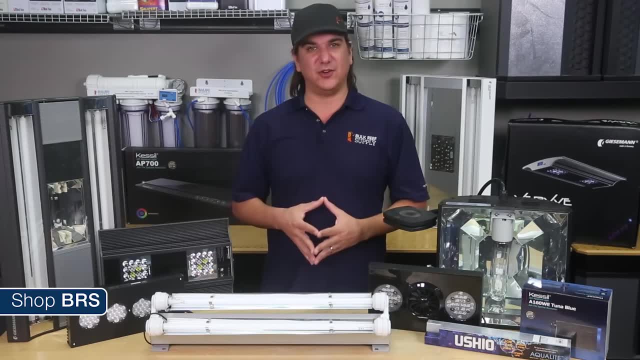 though it might not have matched what you thought. the corals maximum rate of photosynthesis is at the very beginning and end of the day, not in the center, where the peak PAR levels are. it can tolerate more intense PAR levels, but it would certainly appear that PAR is. 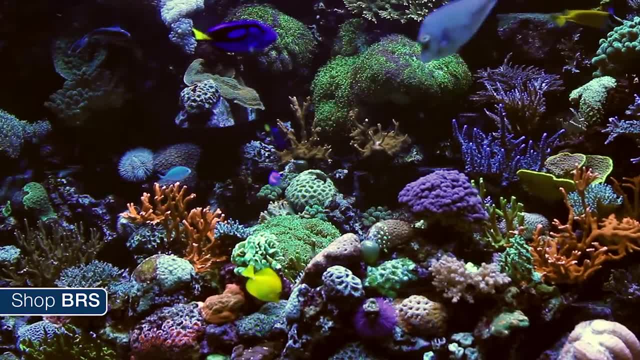 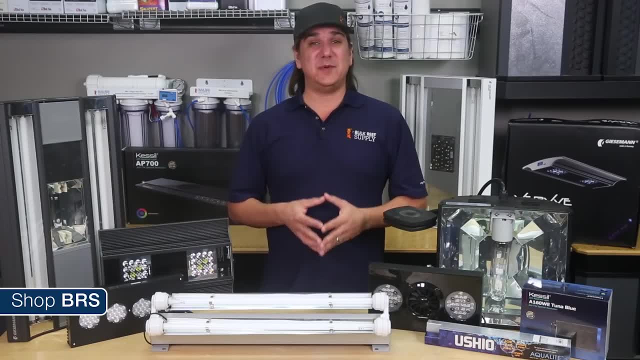 not horsepower, where more is better, and the PAR wars are more of an effect of marketing and selling products than it is about maintaining thriving reef tanks. So what is the right amount? Well, luckily that range seems to be rather large and very accommodating to our needs. 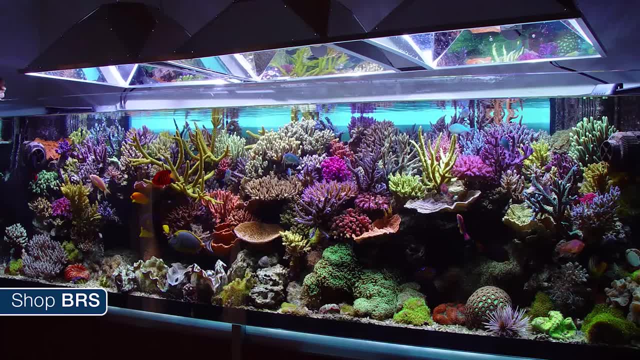 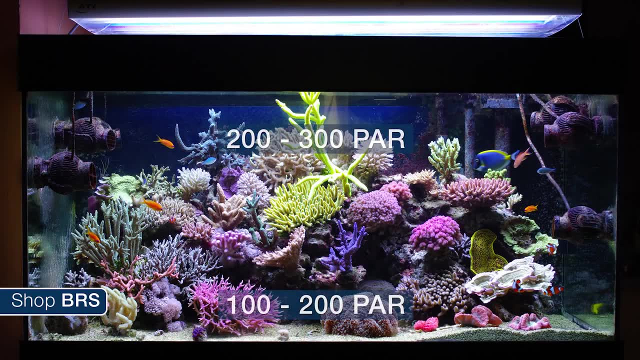 in this case anywhere from near a hundred to into the multiple hundreds. This is likely why reefers had such easy to implement success with SPS corals using a halide, and T5s, which are often in the 100s at the bottom of the tank into the 200-300s. 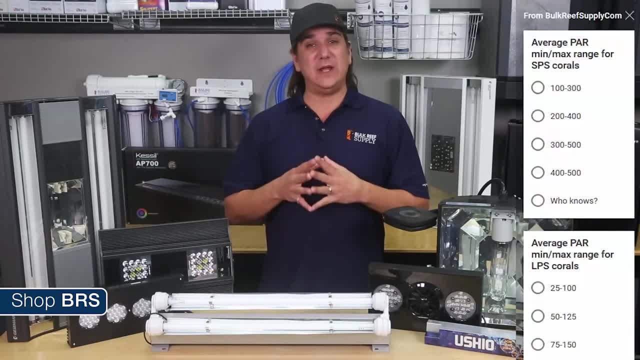 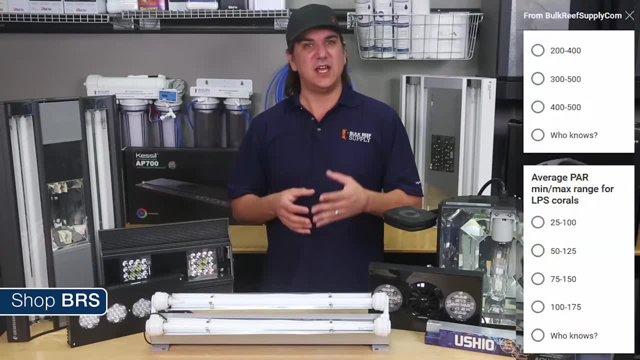 near the top. So this is a critical point where we are just going to ask you, the reefing community, to chime in on what your experience has shown. the top and bottom PAR ranges should be for SPS and LPS tanks using the pole in the upper right hand corner. 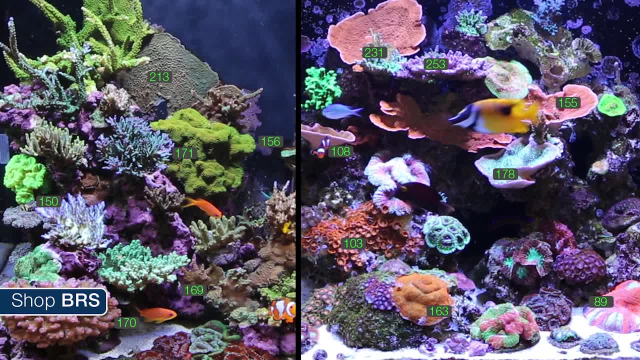 Actual data from successful reef tanks is 100 times more valuable than any theory, so your input is going to be a key component in how we test and evaluate the lights we test in the future. In addition to that, in the upcoming weeks we are going to be talking about the different. 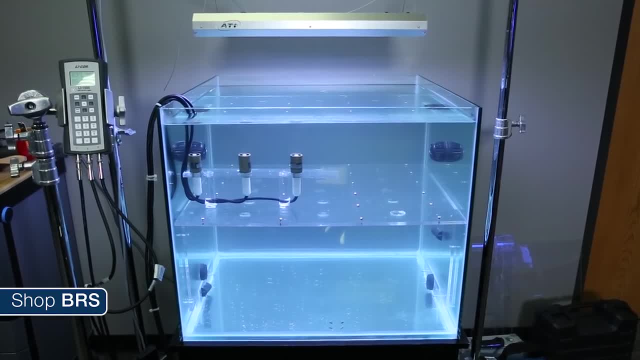 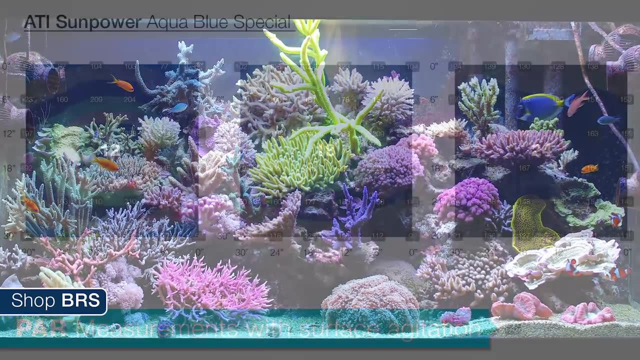 types of reefing and how we test and evaluate the lights we test in the future. In the coming weeks we are going to install and measure some popular reef tank lighting options. the entire reefing community should be able to universally agree has produced very easy to replicate awesome reef tanks and then share those PAR numbers as a baseline. 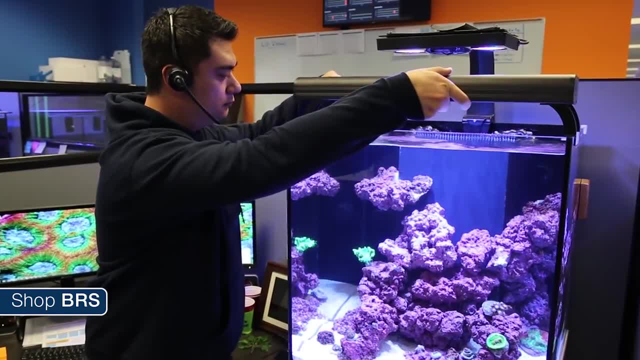 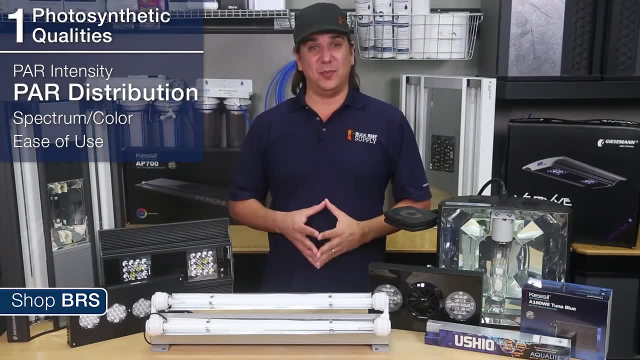 of success. Adventurous reefers and trailblazers can explore results and benefits outside that range, but having a baseline of success is pretty valuable. So in relation to that we move on to the second element of photosynthetic qualities: distribution of that intensity or proper PAR range. 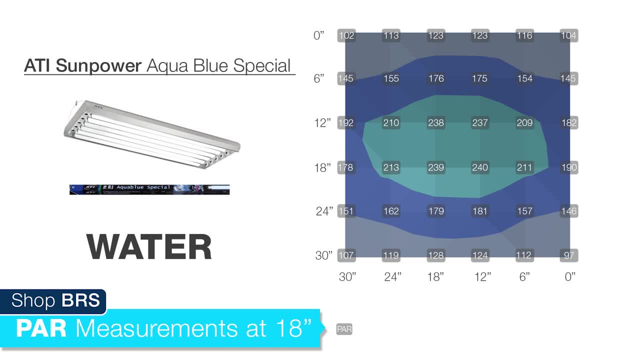 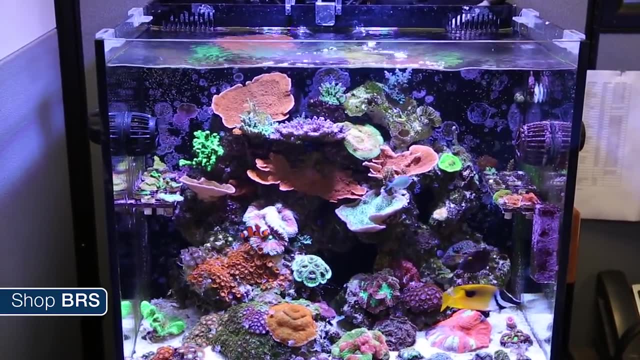 Simply saying PAR is 300 at the top. It really isn't accurate, because each of these light sources distributes the PAR so differently, Particularly in the top half of the tank where a large portion of the corals are. One light source may be fairly even, with mostly 200-300 PAR from left to right and the other 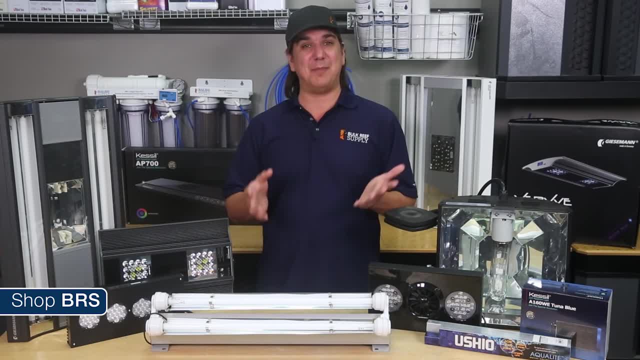 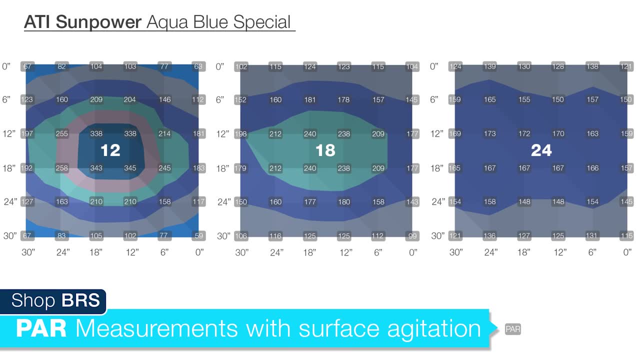 might have a hot spot in the center, 6 inches of 500-600, and then rapidly falls off. For that reason, we are not only going to share peak PAR numbers, but also PAR numbers at multiple depths in a wide grid, and on top of that we plan on giving it to you in multiple tank. 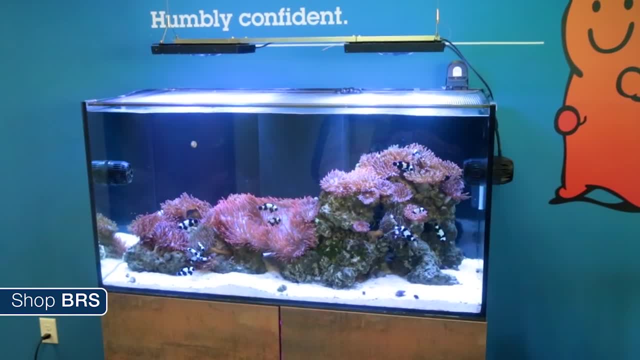 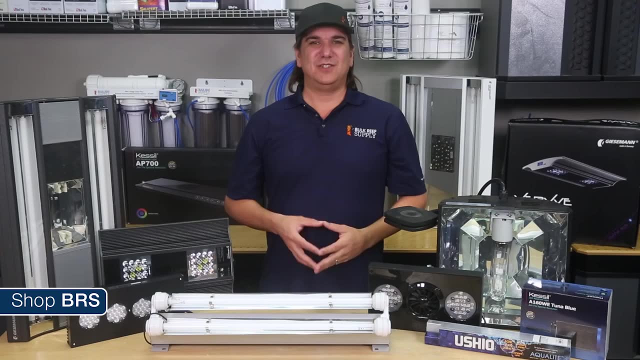 shapes and even with multiple lights, Such as 2-4 of your favorite LED lights, Your favorite LED on a 120, so you can get an idea of how multiple light sources interact with each other when you are planning or perfecting your lighting setup. 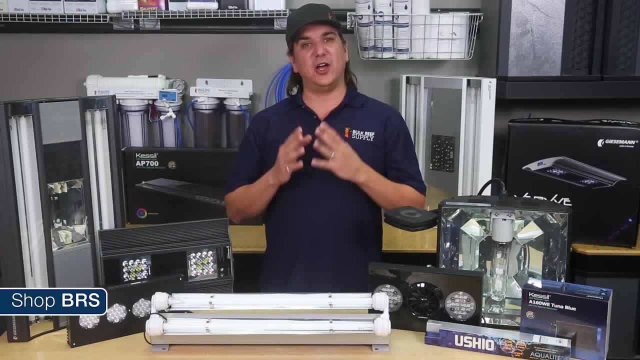 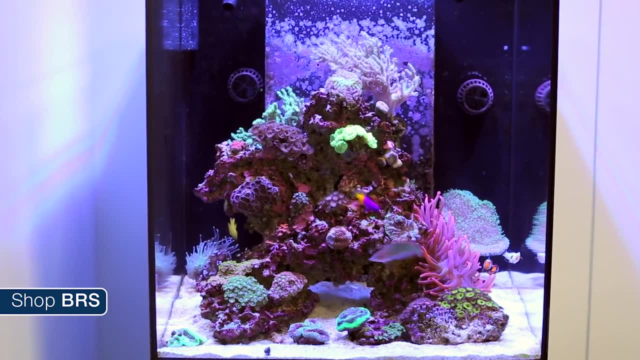 So again, we are asking all of you for your help here. What would be the most valuable to you? Our initial thoughts are: a vast majority of tanks are 24 inches less wide or tall, so a 24 inch cube would be a good environment for measuring most single light sources. 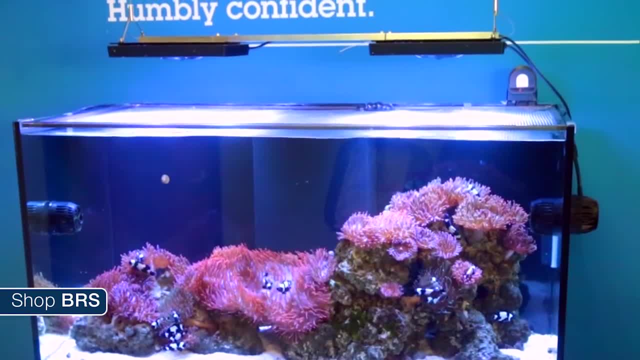 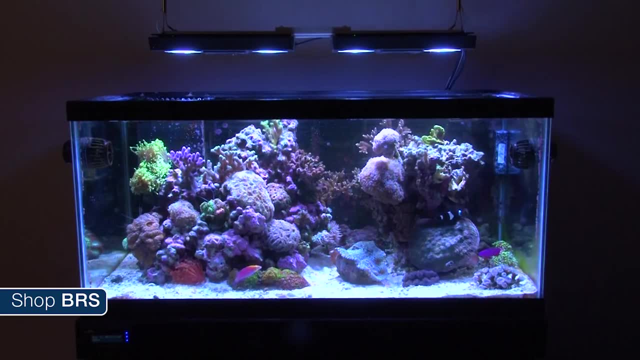 Then, beyond that, measuring multiple of the same light source on a 120 gallon tank, See the difference between running two or three radions, as well as the difference between running them in different orientations And for smaller light sources. doing the same thing on a 40 breeder, which is a very popular. 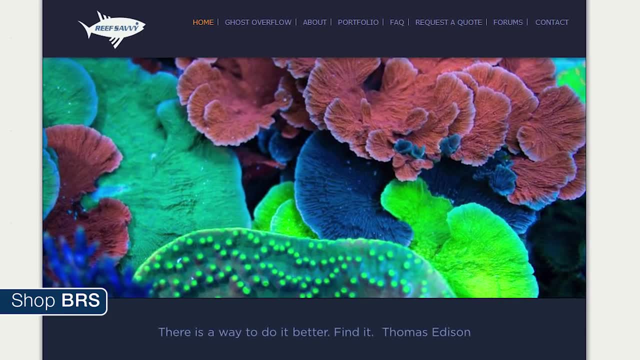 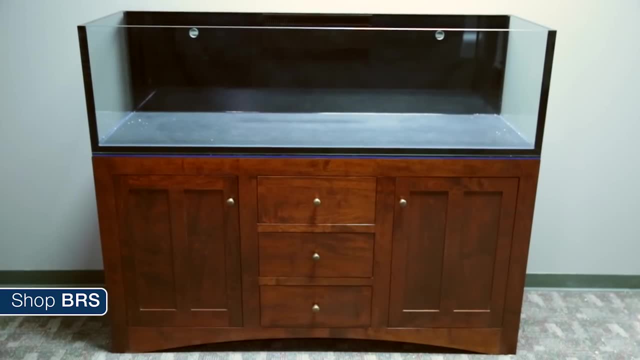 mid-range tank. I already have Felix at Reefs Avenue building us a rimless 120 specifically for this purpose, or Chris at Benner's Woodworking or Sticks and Stones making a stand for us. For those of you that don't know, they are the tank and stand builders from the BRS-116. 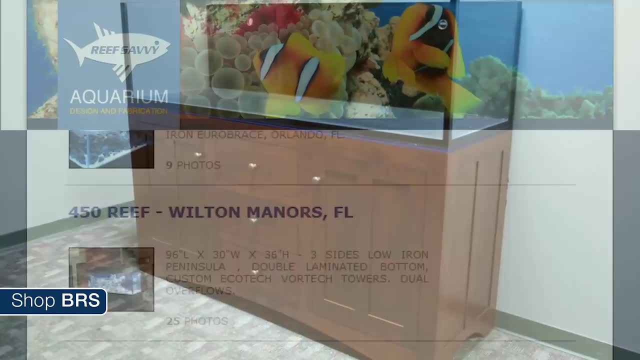 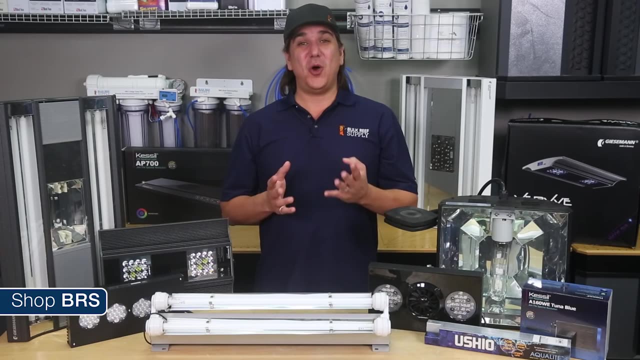 at this point the only custom tank or stand buildings I am willing to use, Felix in particular, has become rather popular, so the wait is pretty significant in most cases, but anything good is worth waiting for. So, knowing we have a tank and stand builder, we are going to take a look at the tank and 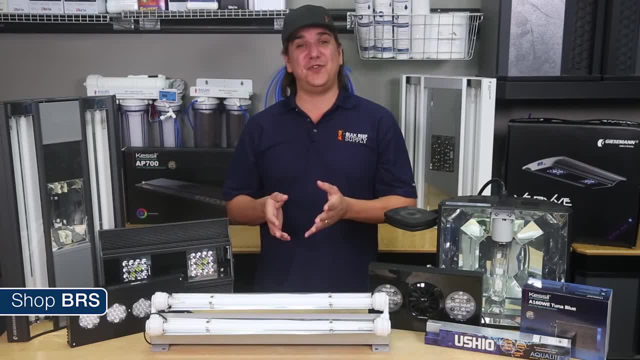 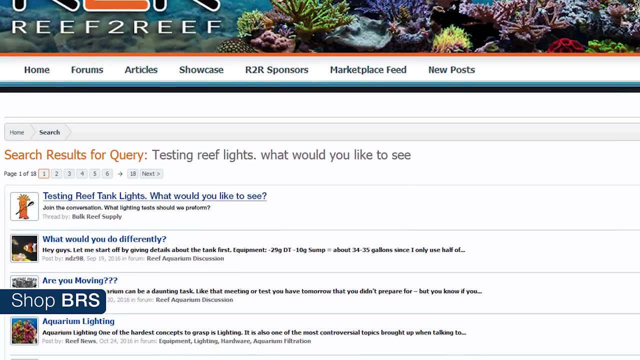 stand builder, If you can't test in every last environment. do us in the community a huge favor and share what you think of the most valuable environments in the comments below, If you would like to take part of a larger discussion on the topic. we are also going. 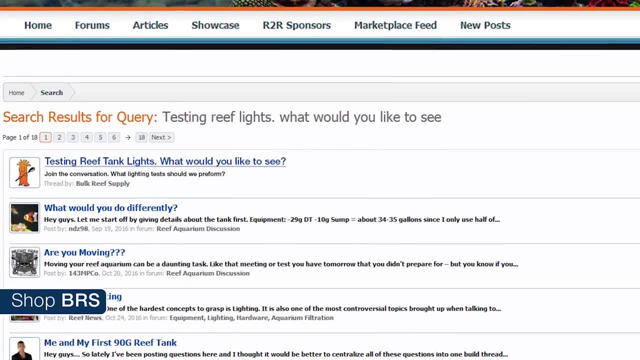 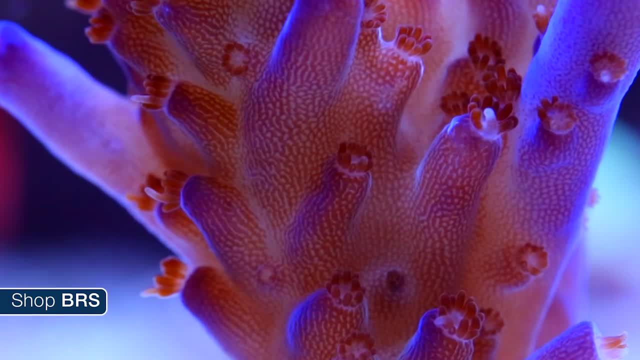 to start a thread on Reef2Reef called testing reef tank lights. what would you like to see? The third component of photosynthetic qualities of light is spectrum. There has been a tremendous amount of talk in relation to spectrum and growth, health and coloration. 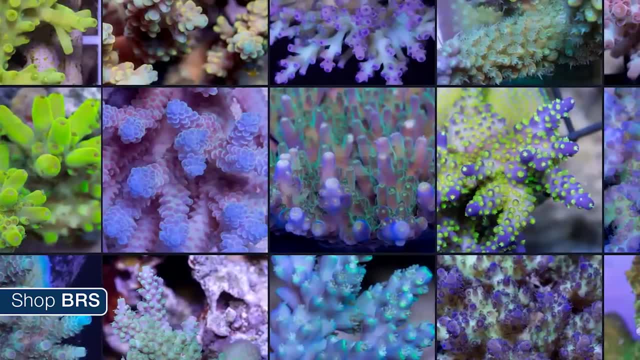 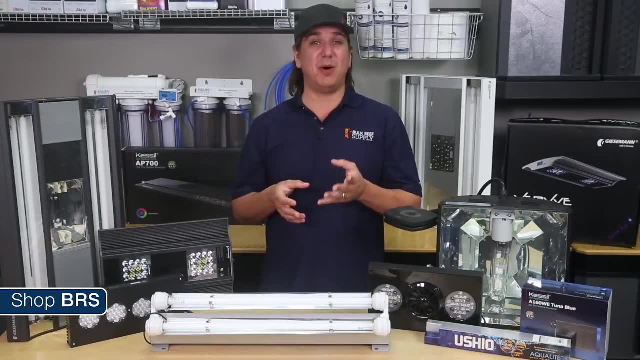 This one is a bit of a mystery to everyone, particularly because we have all seen some pretty incredible results. For example, this is a type of bulb that Adam from Battle Corals uses on his corals, and there is no doubting his results. However, a huge city in the reefing community has also seen tremendous results with blue 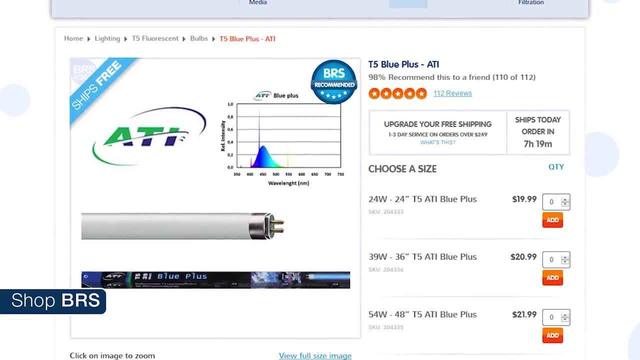 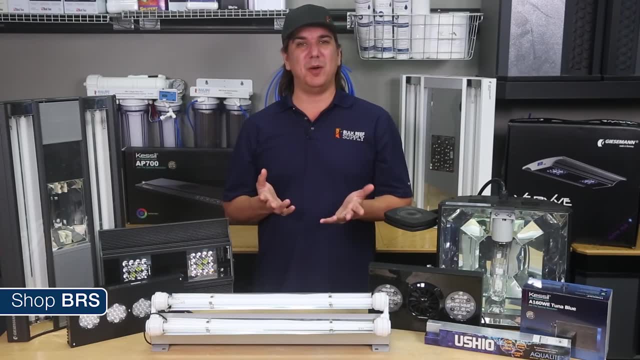 halide bulbs like the radium or blue plus ATI bulb, which is predominantly blue spectrum and closer to what you would find in deeper reefs. So which one is right? Well, clearly they both are, but behind that there likely is some growth in coloration differences. 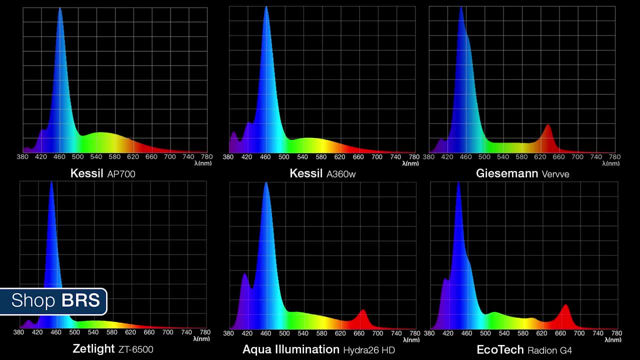 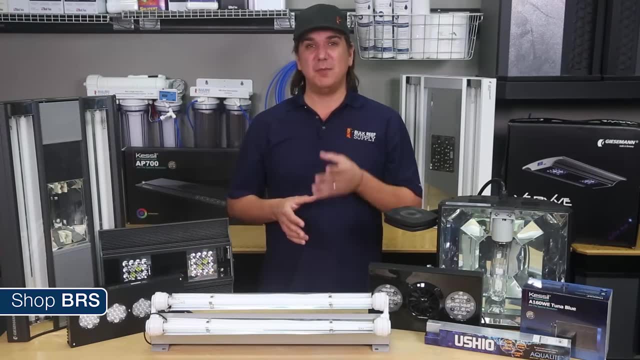 In this series, we will explore what spectrums each light is capable of, What we know in relation to that, as well as the theories presented by the manufacturers of the light, some of which have done some pretty solid research, particularly Ecotec's coral lab and Kessels research. 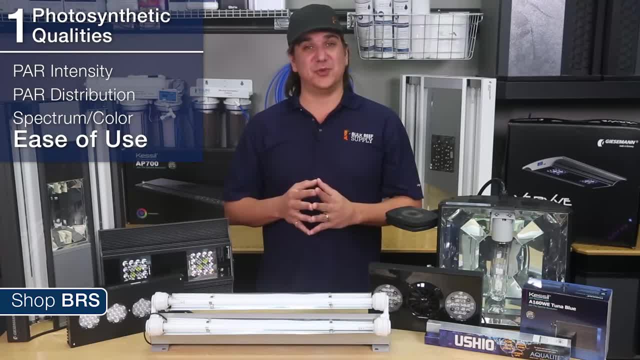 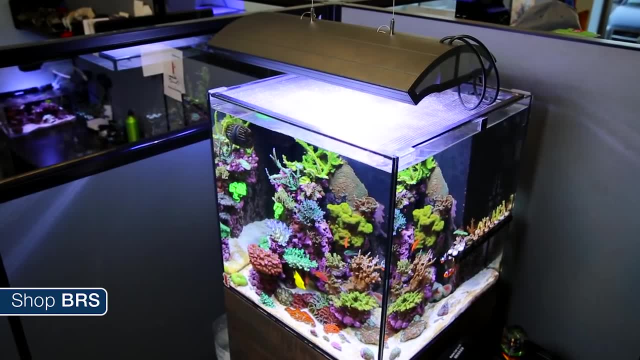 The fourth element of photosynthetic qualities is ease of achieving those results. Frankly, there are a ton of light sources out there where all you need to do is select the right fixture, throw in some popular bulbs and plug it into the wall and you have achieved. 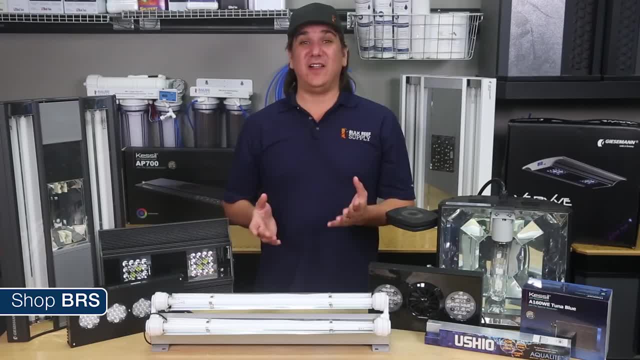 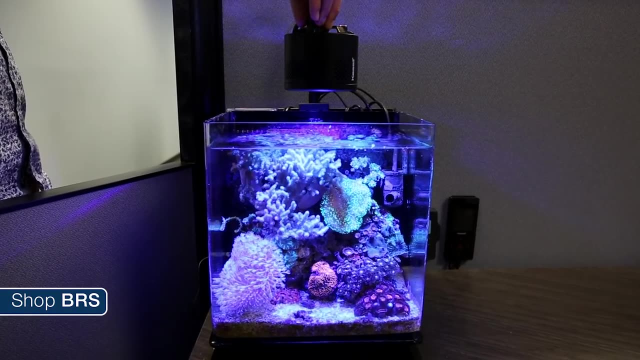 all of the photosynthetic quality goals that we have outlined today. With LEDs that can range from a slightly more complex setup. Extremely difficult to do without significant knowledge of your goals and ways to measure that success. like PAR meters In general, the more compact a light source, the more thought needs to go into proper distribution. 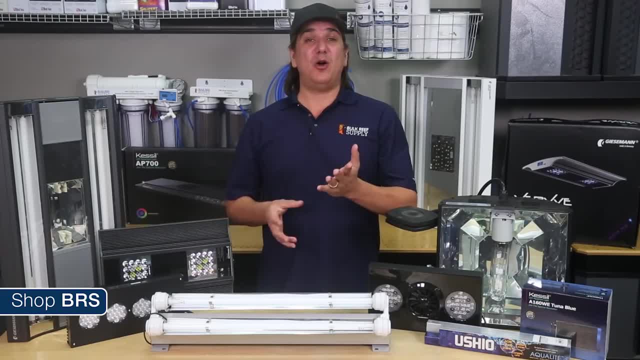 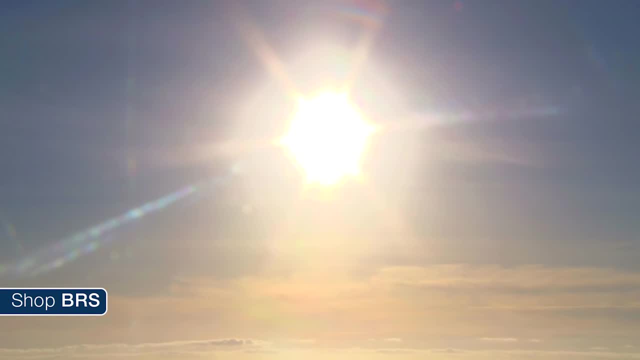 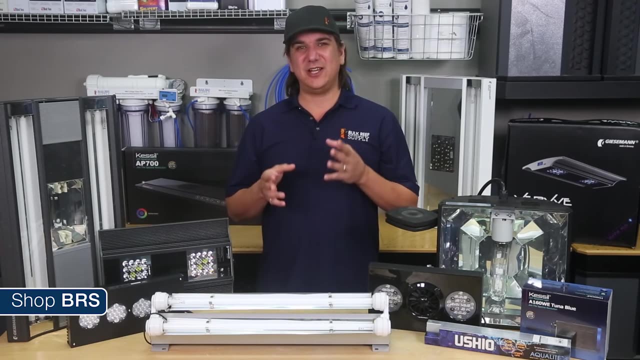 of PAR, particularly at higher ranges. Behind that, the more powerful the light source, the more difficult it is to gauge proper intensities. With a light source capable of achieving mid day natural reef PAR numbers, you have to decide if that is indeed your goal. If you selected a light marketed at working on a 3 to 4 foot deep tank and you only have 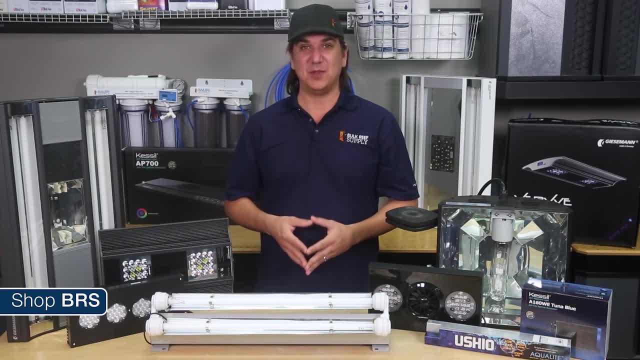 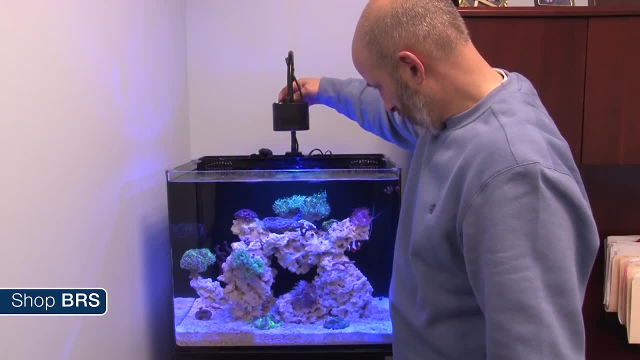 a 2 foot deep tank, You almost certainly need to turn it down drastically. There are also lights which give you the keys to the kingdom on spectrum and those that restrict you to only options known to be good for corals. So we will share our thoughts and how easy it is to achieve photosynthetic results with. 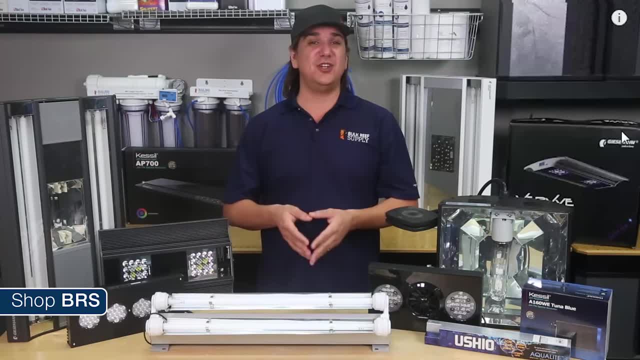 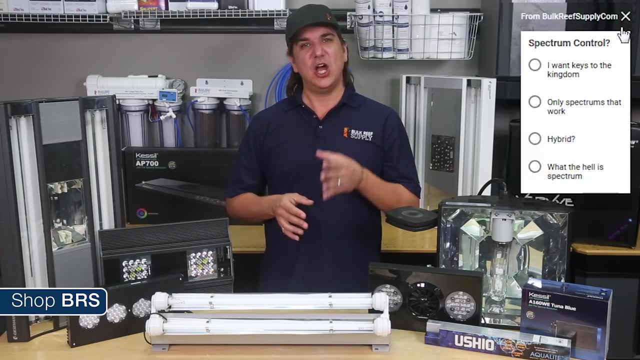 each light source. This is another point where we put up a poll and we would love to know your thoughts. Do you really want the keys to the spectrum kingdom and the ability to adjust every LED to any intensity, Or would you prefer the lights were locked down to spectrum mixes, which are known to 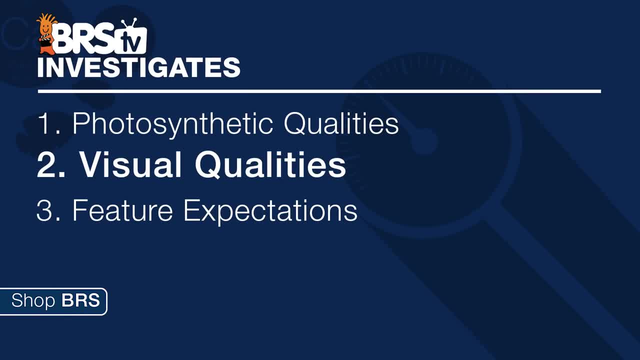 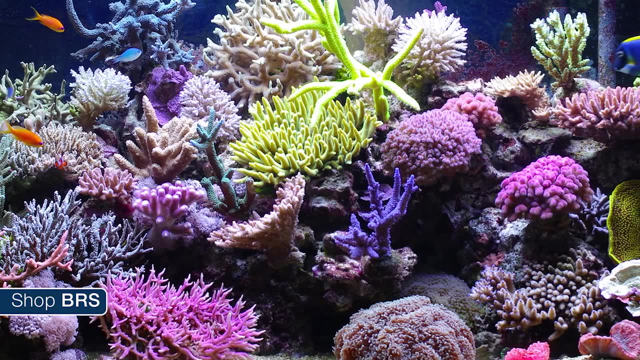 produce the best results. So, moving on, the second major element group that we are going to talk about is visual qualities. Right after keeping corals healthy, the most significant factor for most reefers is how does the light make the corals and tank look? 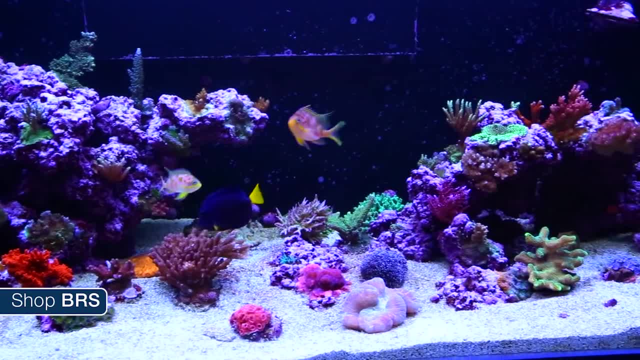 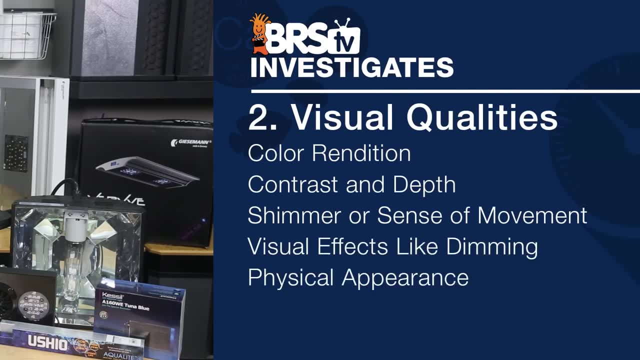 At the end of the day, we want the tank and corals to look awesome, and this is a primary reason most of us have reef tanks in our homes. to begin with, There are 5 elements. we will review visual qualities for color rendition, contrast and 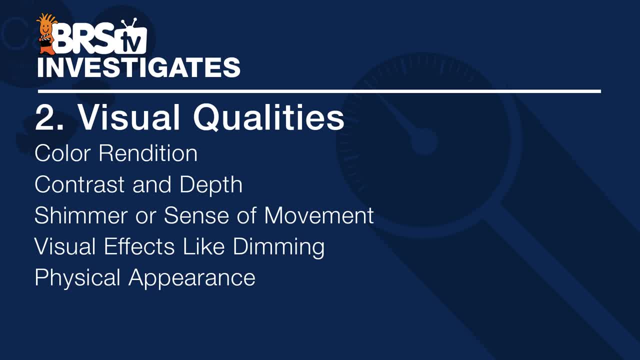 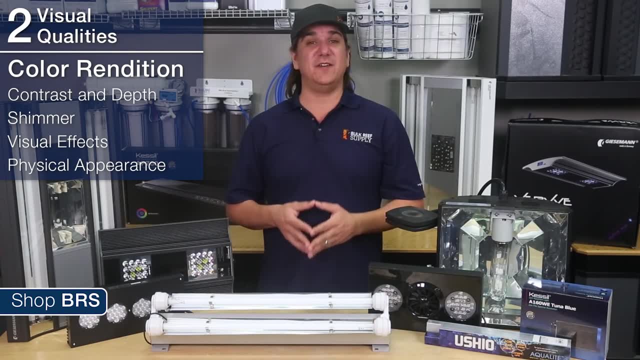 depth, shimmer or sense of movement, visual effects like dimming and the physical appearance of the light source itself, Number one being color rendition is primarily limited to the available bulbs or types of LEDs included in the light, as well as the controls over how the spectrum mix works. 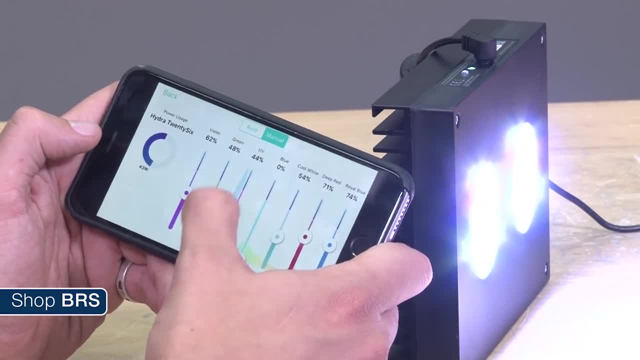 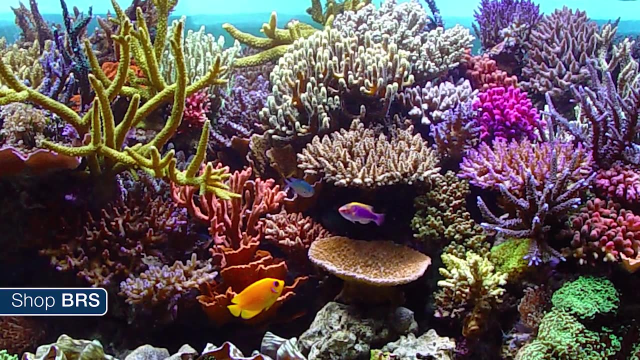 There are some pretty huge differences between various light sources in this regard. Second, contrast and depth is something a lot of reefers who aren't professional photographers overlook. However, this is the type of lighting which often gives the most impactful visual appeal to the reef tank. 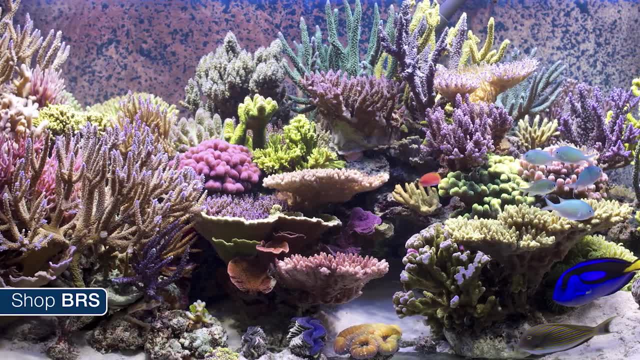 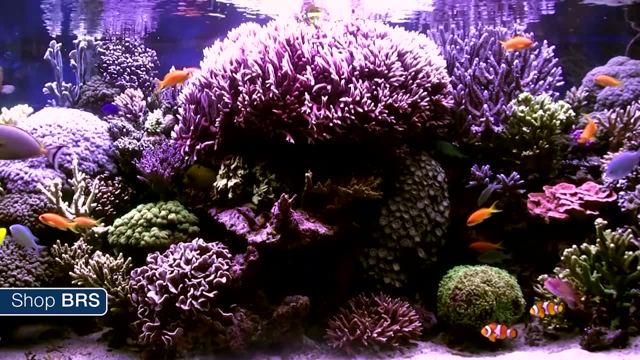 Sometimes the best PAR distribution, which creates a flat blanket of even light, is inherently at odds with contrast and sense of depth, where some areas of the tank are intentionally darker or shadowed to create contrast and visual appeal. We'll share how the light performs in that regard as well. 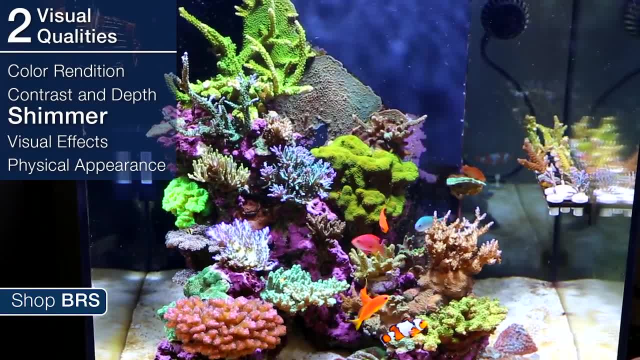 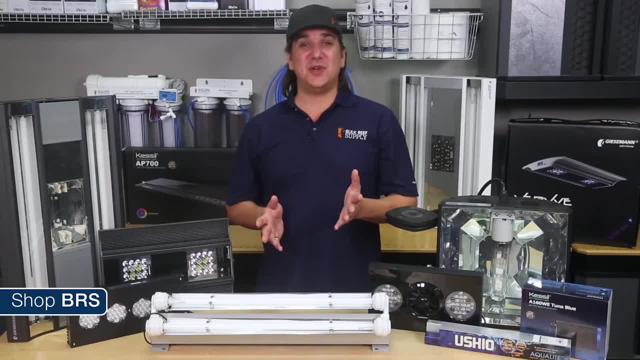 Third is a visual shimmer that transforms what often looks like a photograph of a reef into a section of a living reef in your home. Halides are likely the undisputed king in this regard. LEDs also do a nice job, but can have a significant amount of color separation, or what many people 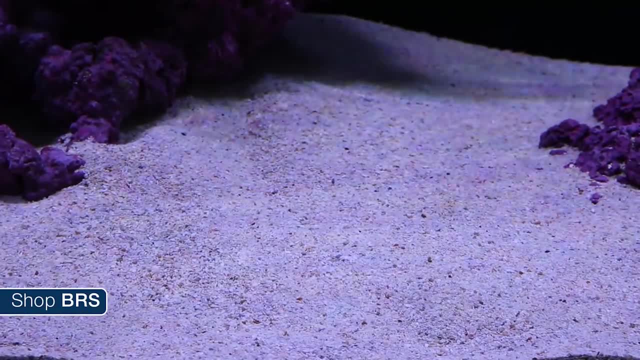 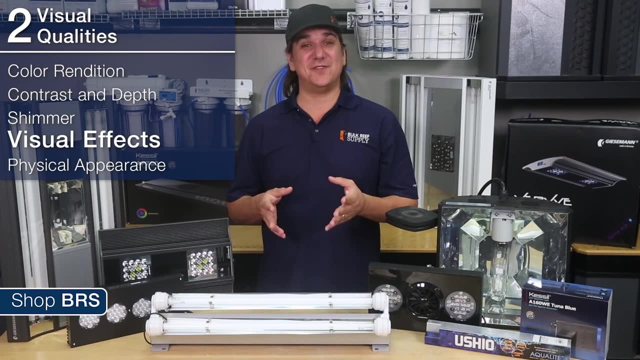 feel is an overpowering amount of shimmer, often referred to as a disco ball effect. We'll share how these lights perform in that regard as well. Fourth being visual effects like dimming, sunset and sunrise effects and moon lights, which absolutely add visual interest to the tank. 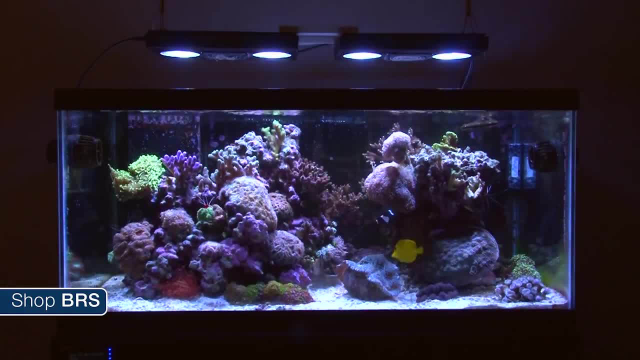 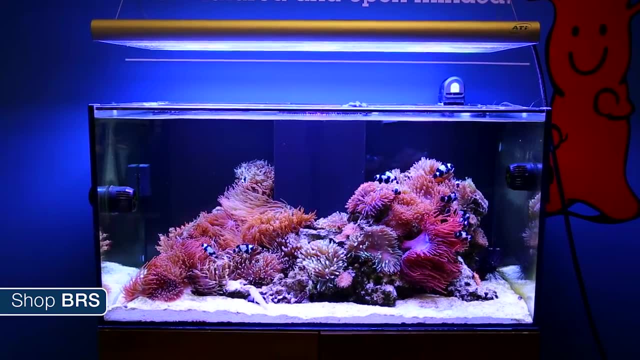 LEDs obviously do this type of thing better than others, but we'll certainly look into who does them the best. The fifth and last quality we'll plan on reviewing is the visual appeal of the light itself. Everyone has a different opinion on this, as well as their willingness to spend money or 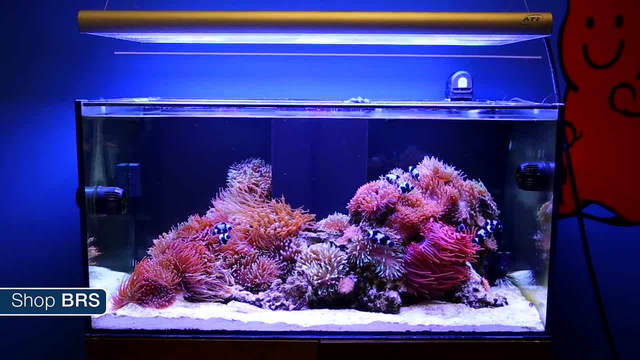 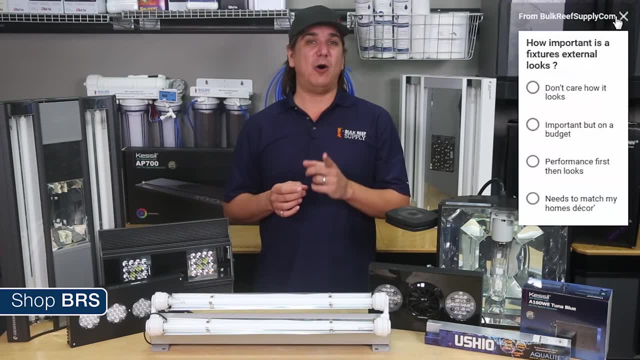 sacrifice performance elements in favor of an appealing fixture or module design. For me, the entire tank needs to look sharp inside and out, But this is the topic of our last poll. How important is the visual appeal of the light fixture itself, specifically in relation to performance and price?